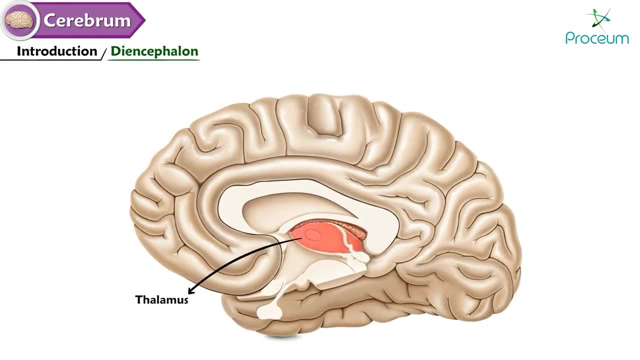 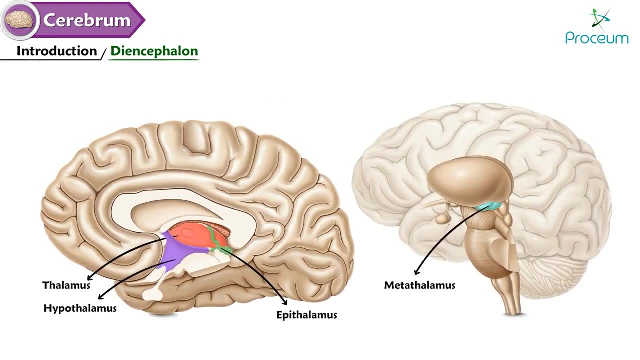 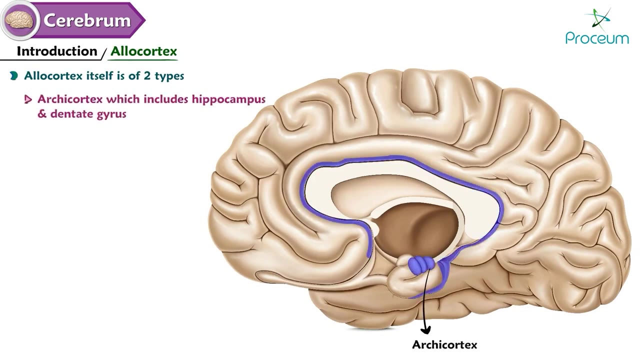 Diencephalon Consists of the thalamus, hypothalamus, epithalamus and metathalamus. Now let's talk about the cerebrum in detail: Allocortex. Allocortex itself is of two types: Archicortex or archicortex. 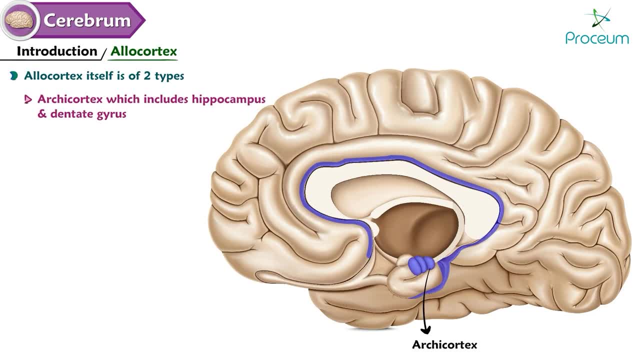 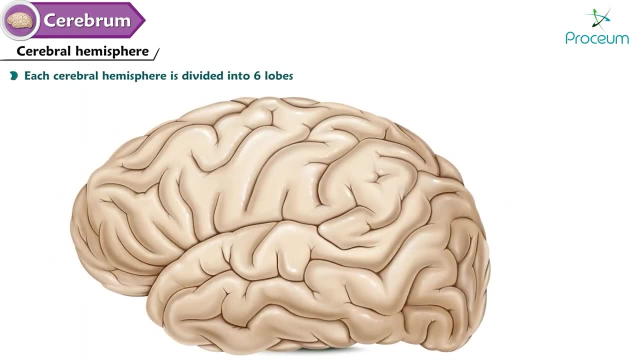 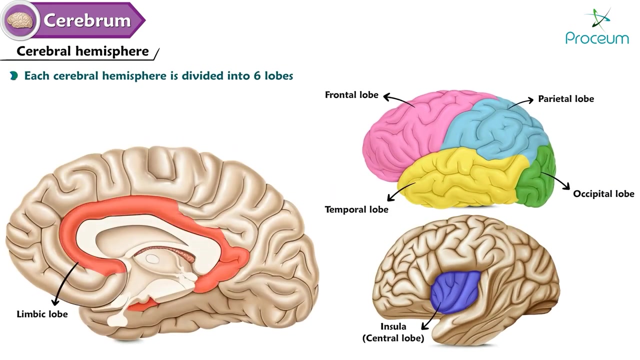 Archicortex, which includes the hippocampus and the dentate gyrus. Paleocortex, which includes the olfactory cortex Cerebral Hemisphere. Each cerebral hemisphere is divided into six lobes. They are Among two cerebral hemispheres. one is dominant by its function, such as language. 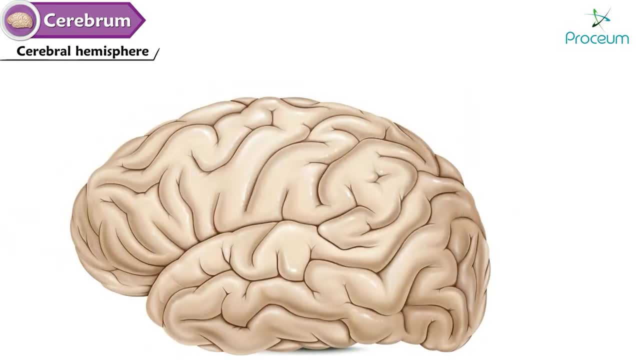 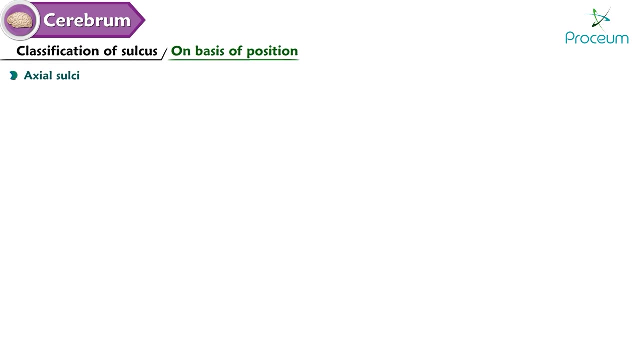 speech comprehension. The cerebrum is full of grooves and ridges running in every direction. These are called sulci and gyri respectively. On the basis of position. there are four types of sulci: Axial sulci. Some sulci develop along the axis of a rapidly growing or developing area. 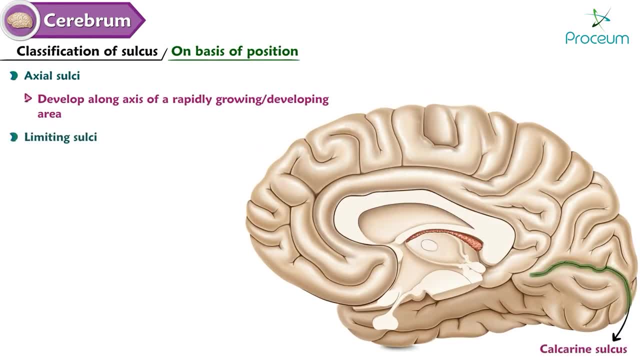 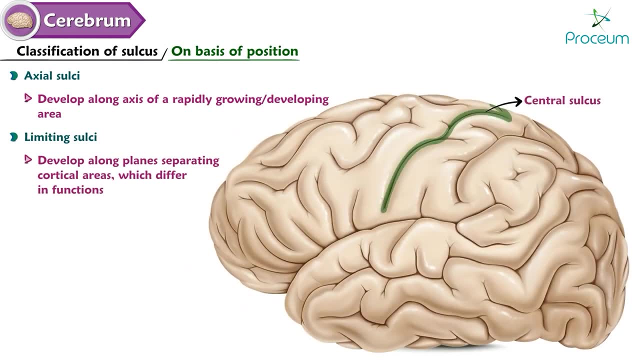 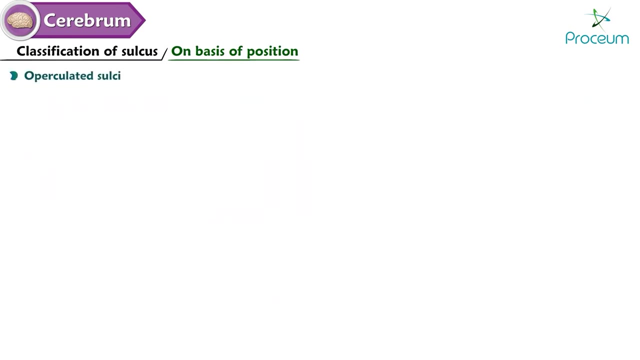 Example: calcarine sulcus. Limiting sulci develop along the planes separating corticosteroids. These are the typical areas which differ in functions. Example: central sulcus which separates frontal motor cortex from the parietal sensory cortex, Operculated sulcus. 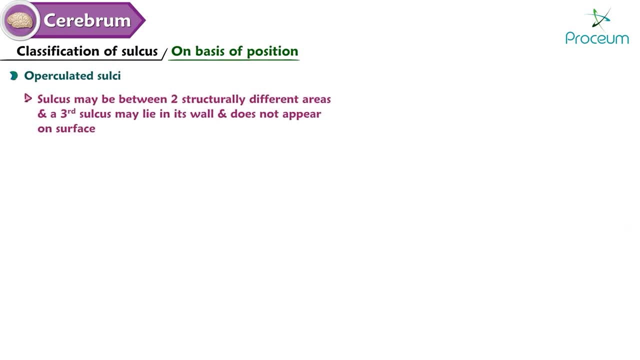 A sulcus may be between two structurally different areas and a third sulcus may lie in its wall and does not appear on the surface. For example, lunate sulcus, Complete sulcus, is deep enough to produce an elevation in the wall of a ventricle. 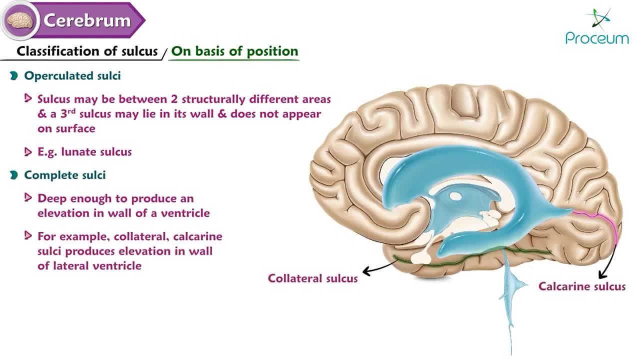 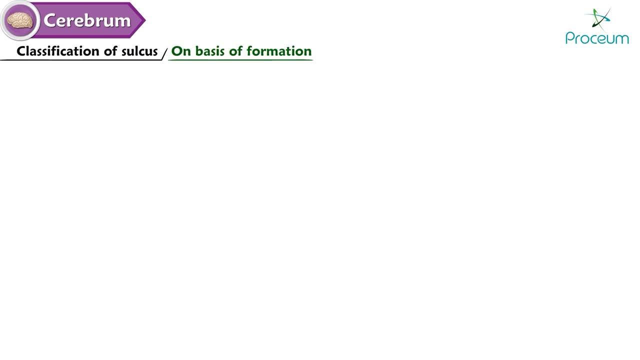 For example, a colorectal sulcus, Collateral calcarine sulci, produces elevation in the wall of lateral ventricle On the basis of formation. there are two Primary sulcus formed before birth, For example central sulcus. 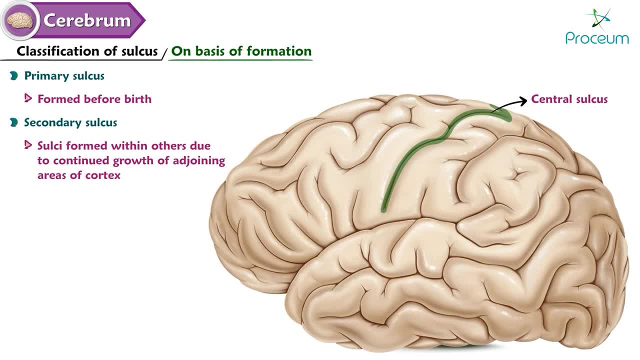 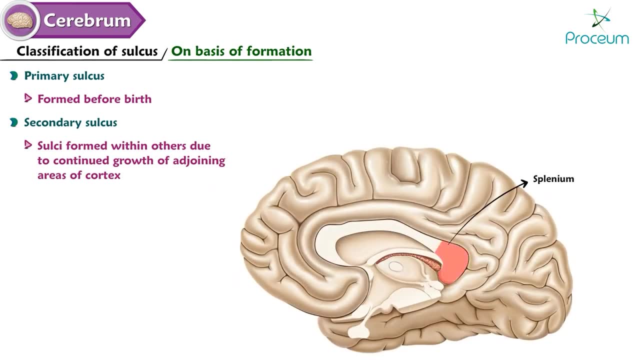 Secondary sulcus, sulci formed within others due to the continued growth of adjoining areas of cortex. Example: the splenium of the corpus callosum conveys a large number of fibers from the temporal and occipital To the parietal occipital sulcus, creating a number of axial and limiting sulci within the wall of the parietal occipital sulcus. 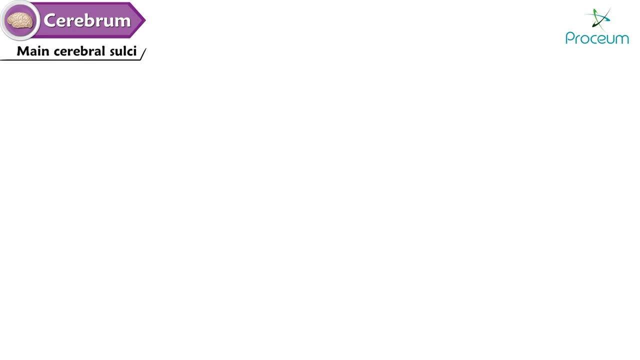 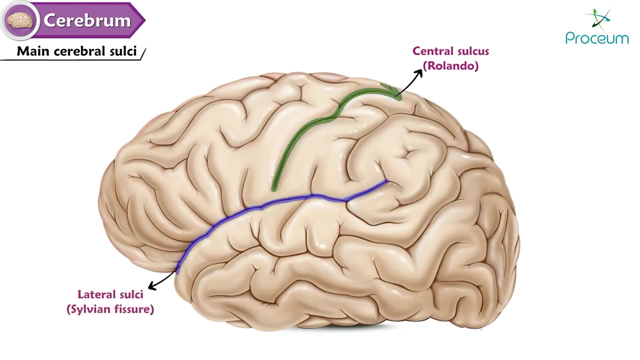 Let's take a look at the main cerebral sulci. Central sulcus of Rolando separates the frontal and parietal lobes. Lateral sulcus, also known as Sylvian fissure, separates the frontal and temporal lobes anteriorly. 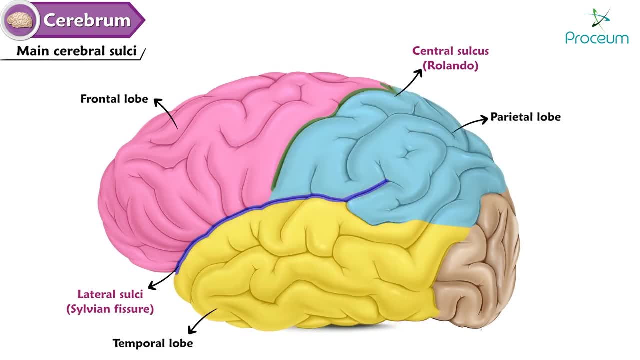 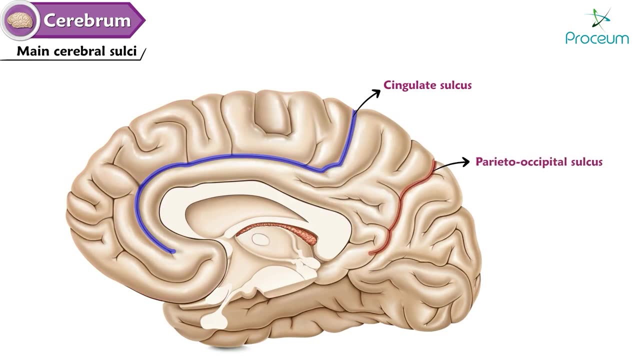 And the parietal and temporal lobes posteriorly. And the parietal and temporal lobes posteriorly. Singulate sulcus separates the cingulate gyrus from the frontal and parietal lobes. Parietal occipital sulcus separates the parietal and occipital lobes. 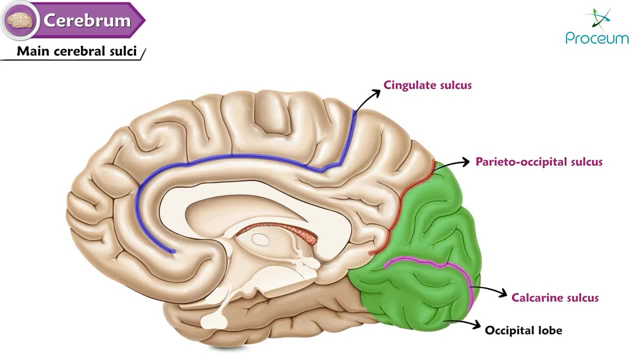 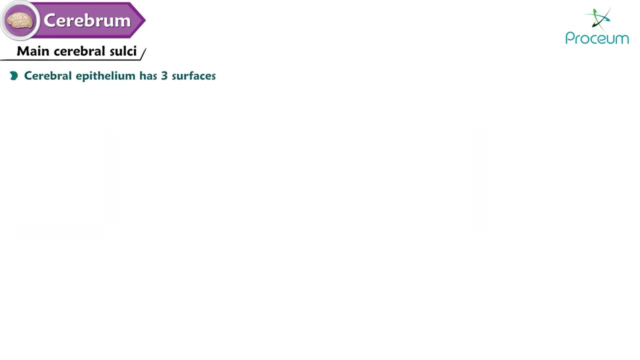 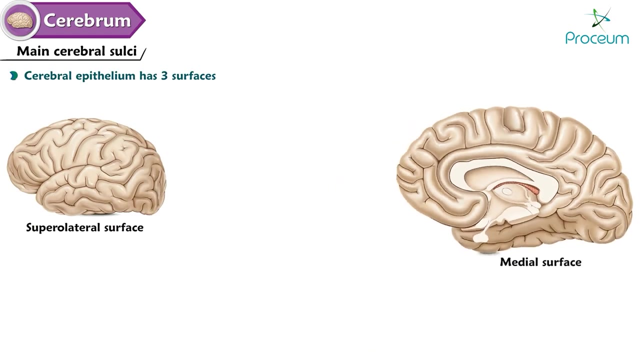 Calcarine sulcus divides the occipital lobe horizontally into cuneus superior and lingual inferior gyrus. Cerebral epithelium has three surfaces. They are superior, lateral surface, medial surface, inferior surface, superior surface, which has orbital and tentorial surface. 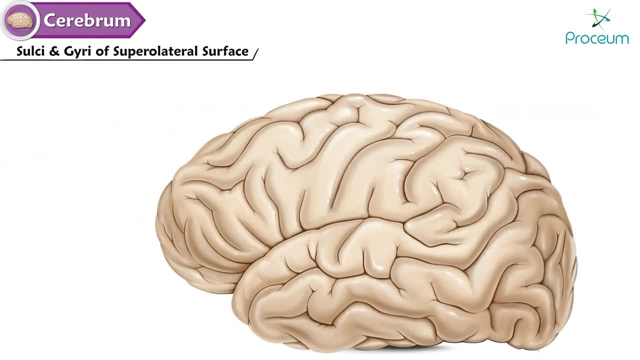 Sulci and gyri of superior lateral surface of cerebrum. Following are the sulci and gyri of the frontal lobe: Sulci: precentral sulcus. superior frontal sulcus. inferior frontal sulcus. lateral sulcus Gyri- precentral gyrus, superior frontal gyrus, middle frontal gyrus. 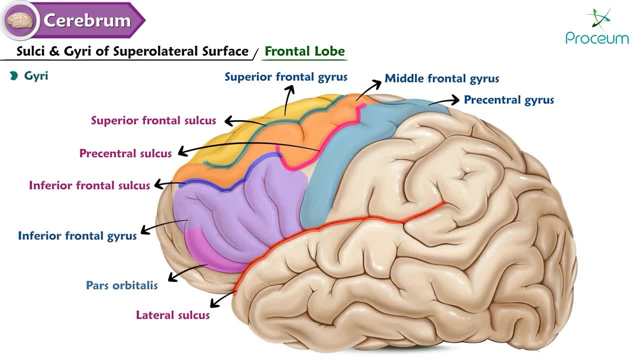 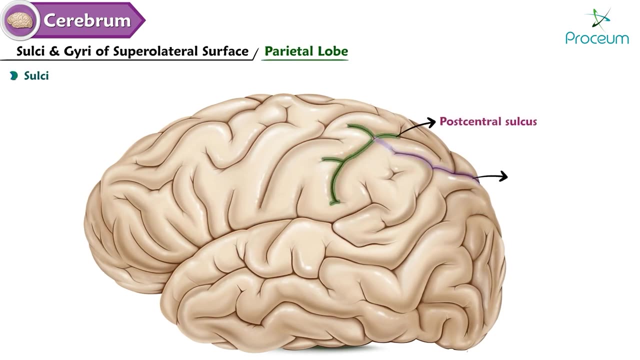 inferior frontal, which is divided into pars orbitalis, pars triangularis and pars opercularis. Following are the sulci and gyri of the parietal lobe. Sulci are as follows: Postcentral sulcus, intraparietal sulcus, upturned. end of posterior ramus of lateral sulcus. 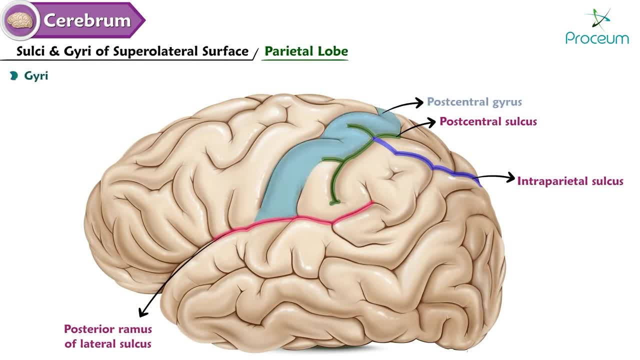 Gyri postcentral. gyrus superior parietal lobule. gyrus Inferior parietal lobule. gyrus Inferior parietal lobule divided into supramarginal angular and arcus temporo occipitalis. 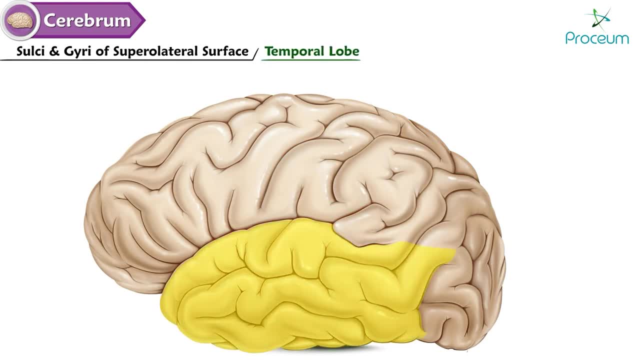 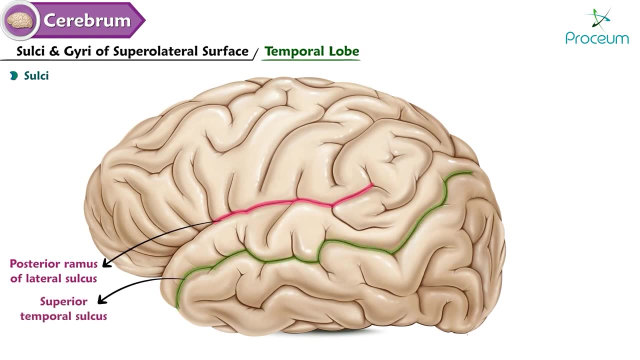 Following are the sulci and gyri of the temporal lobe: Sulci, posterior ramus of lateral sulcus, superior temporal sulcus and inferior temporal sulcus. The gyri are superior temporal gyrus, middle temporal gyrus, inferior temporal gyrus. 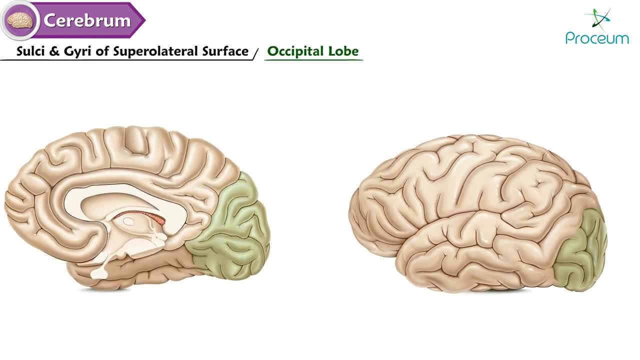 Following are the sulci and gyri of the occipital lobe: Sulci, transverse occipital sulcus, lateral occipital sulcus, lunate sulcus and calcarine sulcus, Gyri, arcus, parietal occipital gyrus, superior occipital gyrus and inferior occipital gyrus. 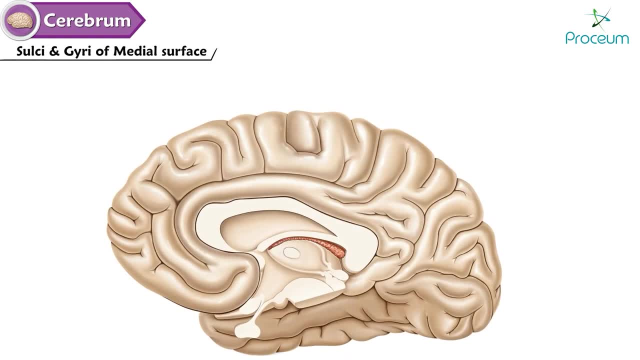 Sulci and gyri of medial surface of cerebral hemisphere: Sulci callosal sulcus, cingulate sulcus, anterior and posterior par-olfactory sulcus, suprasplenial sulcus, parietal, occipital sulcus, calcarine sulcus. 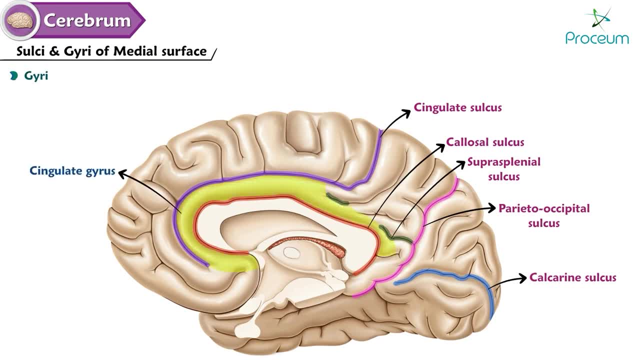 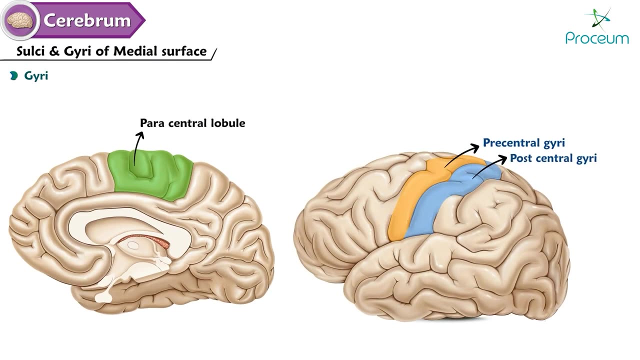 Gyri, cingulate gyrus, medial frontal gyrus, paraterminal gyrus, para-olfactory gyrus and parietal frontal gyrus. Cunus precunus- Paracentral lobule is the continuation of precentral and postcentral gyri on medial surface. 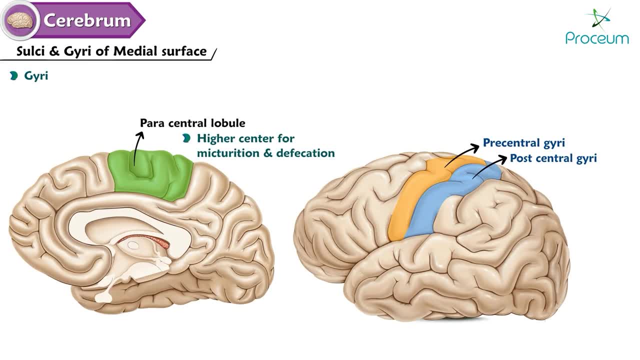 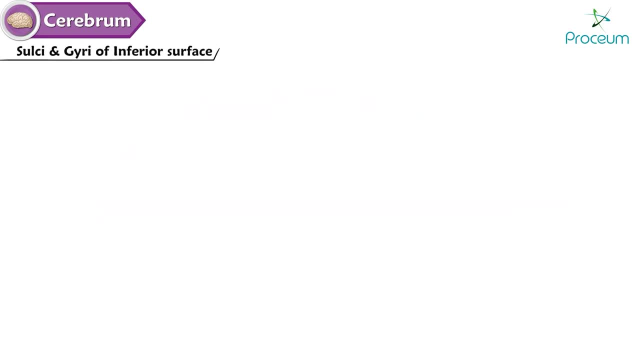 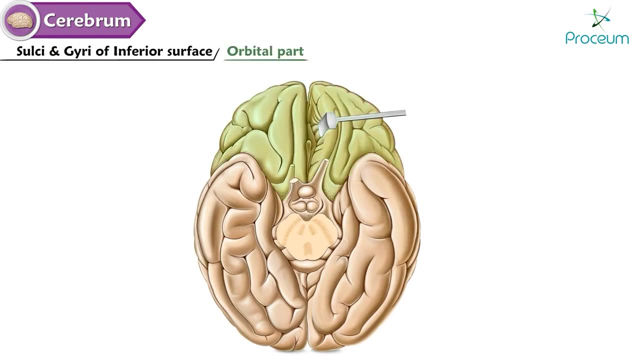 is higher center for mixturation and defecation. Isthmus is the narrow region between splenium and calcarine sulcus, Sulci and gyri of inferior surface of cerebral hemisphere. Following are the sulci and gyri of the orbital part. 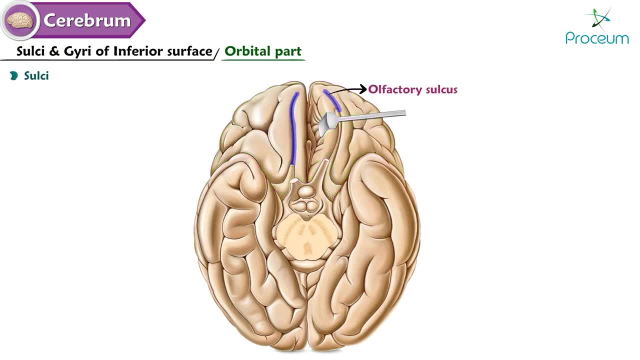 Sulci, Olfactory sulcus, orbital sulcus, lateral sulcus, gyri, Gyrus rectus, medial orbital gyrus, lateral orbital gyrus, anterior orbital gyrus and posterior orbital gyrus. Following are the sulci and gyri of the tentorial part. 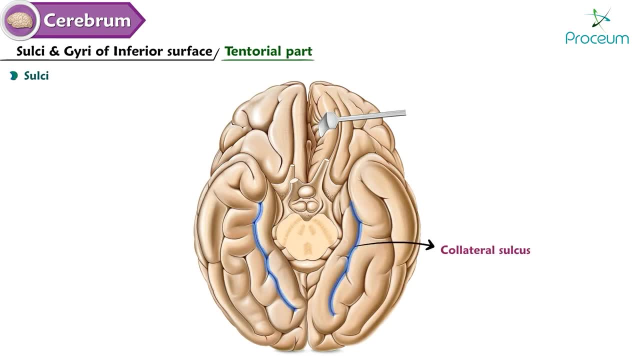 Sulci: Collateral sulcus medial Occipitotemporal sulcus lateral. Rinal sulcus gyri Medial occipitotemporal gyrus lateral occipitotemporal gyrus uncus. 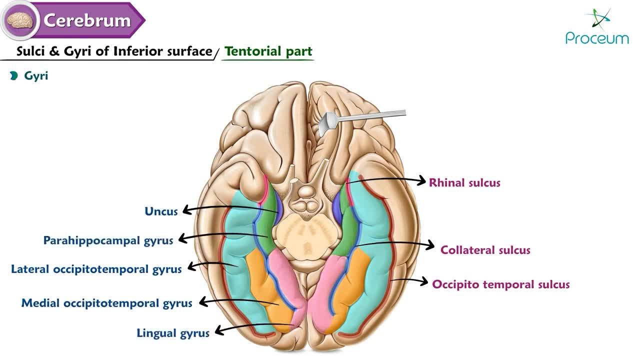 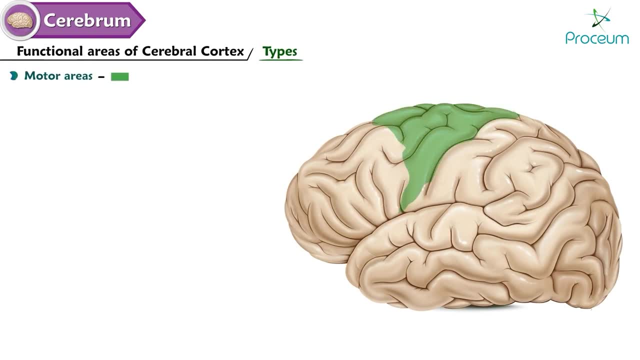 Parahippocampal gyrus, lingual gyrus, Functional areas of cerebral cortex. Types of functional areas are: Motor areas, chiefly concerned with motor activities, give rise to pyramidal tracts. Sensory areas are chiefly concerned with sensory functions. 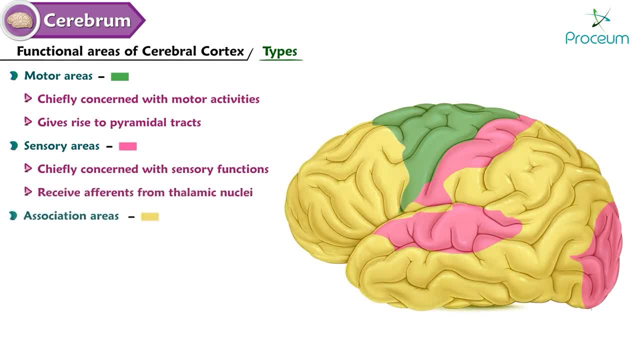 and receive efference from thalamic nuclei. Association areas are neither motor nor sensory, but concerned with integration, association and cognitive functions. Approximately 75% of cerebral cortex is made of association areas. 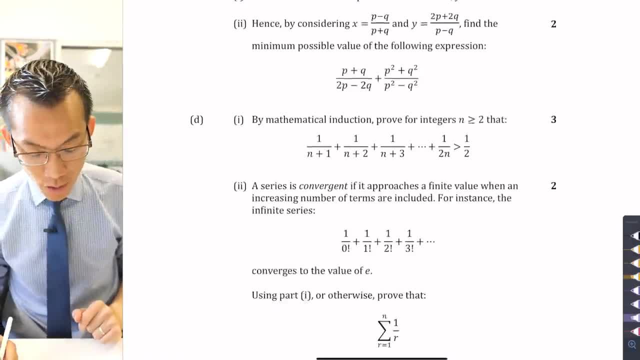 Okay, we are on the final page. Well done for staying with me this long if you've been working all the way through it. This question here wasn't meant to be too arduous if you read it carefully, but a lot of people got quite confused, so let's have a look at the 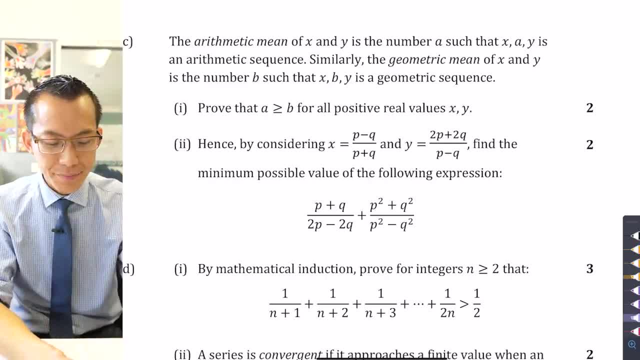 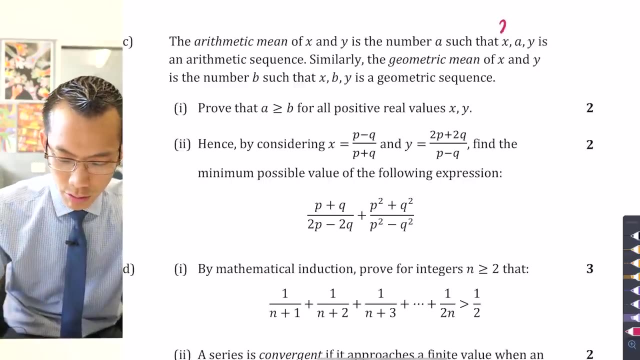 language that's being used and make sure we know what's going on. The arithmetic mean of x and y is the number a, such that x a, y is an arithmetic sequence. Okay, think about this for a second. If I were to present to you two numbers like 2, 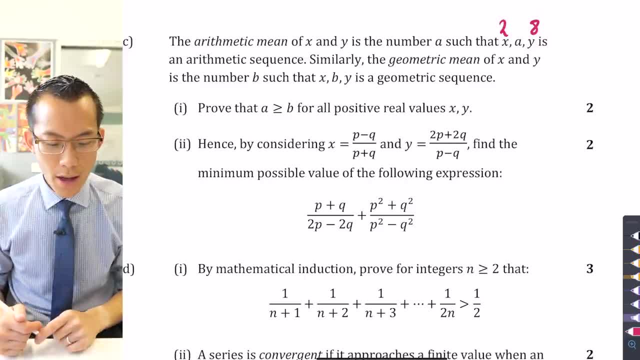 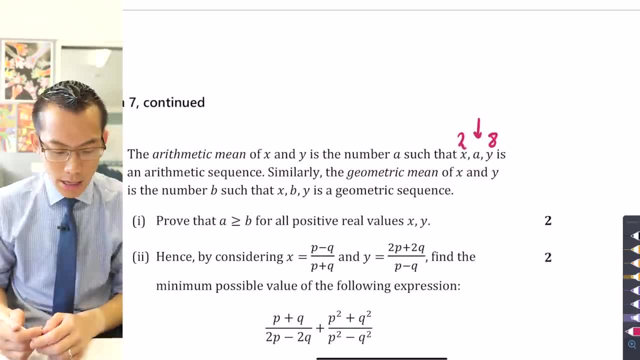 and say 8, x and y, and they're on both ends right. The arithmetic mean of 2 and 8 is the number such that if you stick it in here, you put it in place of a, then you should get an arithmetic sequence. So what number should I put in there that would give me a? 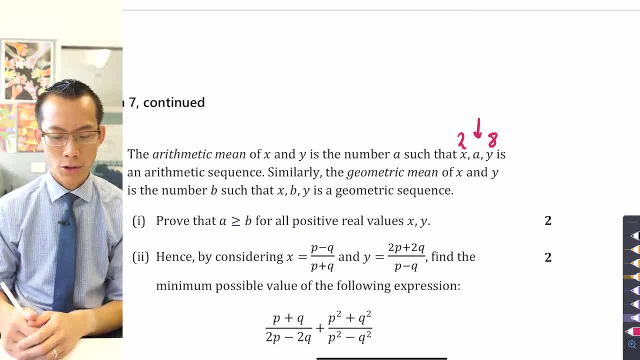 common difference all the way along. That's what defines an arithmetic sequence, after all. Hopefully, your arithmetic is not failing you and you're going to be able to solve it, You realize? oh, it's going to be a 5, right. That gives me a common difference of 3.. So 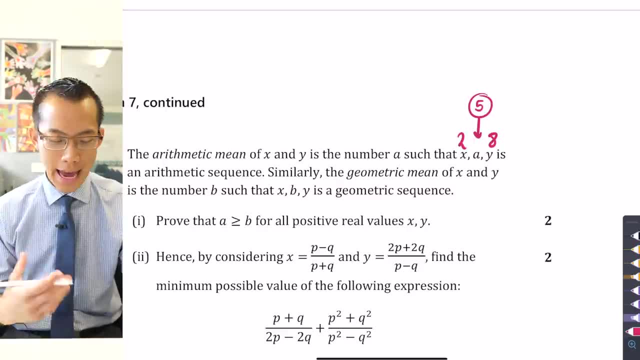 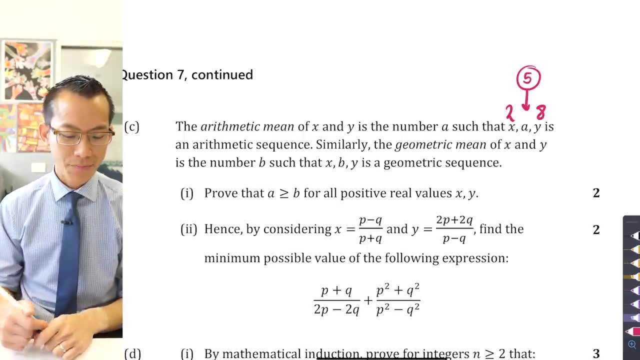 5 is the arithmetic mean of 2 and 8. And we would normally call that the average right. So this is just a fancy name for that, because, as we're introducing you in this question, the arithmetic mean is not the only kind of mean. 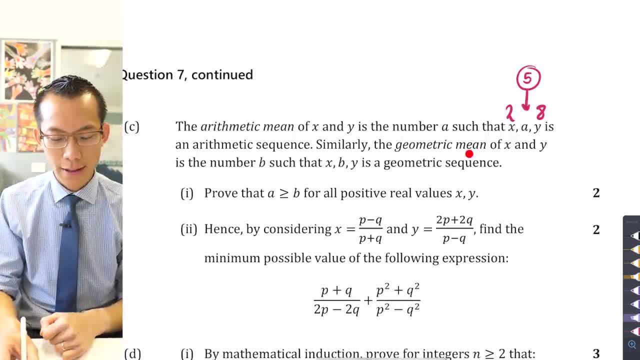 There is also this other term here, the geometric mean. You can have a different mean for x and y, the same two numbers like 2 and 8,, such that x and then your geometric mean b and then y is a geometric sequence. So if I go back to 2 and 8, what's the number?